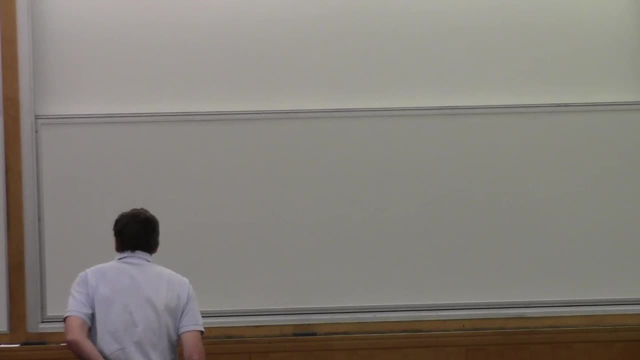 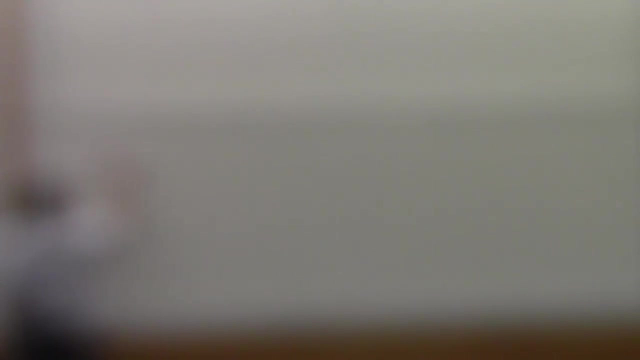 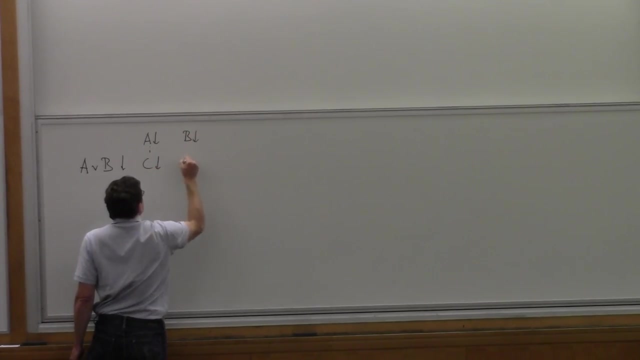 Ah, good question. Okay. So the question was if I have a rule like this: if A or B I can use, that, assuming A I get to use C, then I'm allowed to use C, And this was our alternative version of or elimination. Okay. 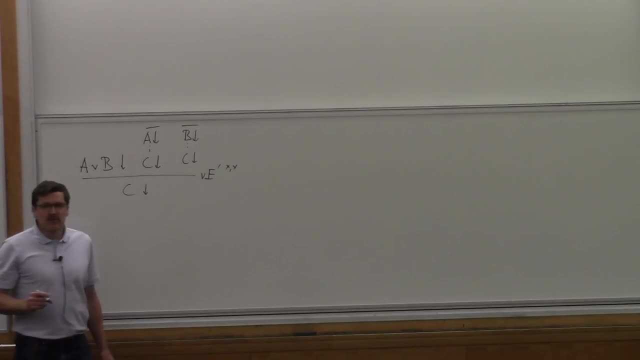 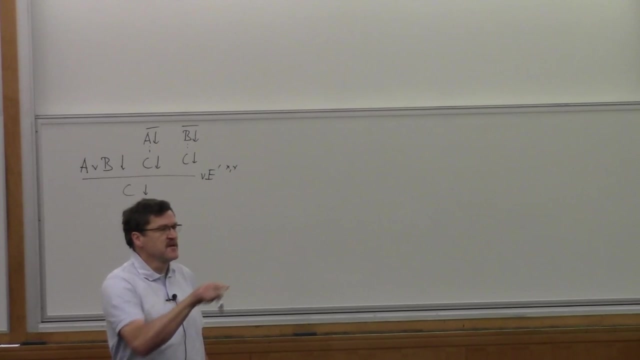 And the question is: the question was: what is the sequent calculus rule that corresponds to that? look like: Okay, Any, any thoughts? Anybody look at this problem. So we have two people who worked on it, Sylvia and me. 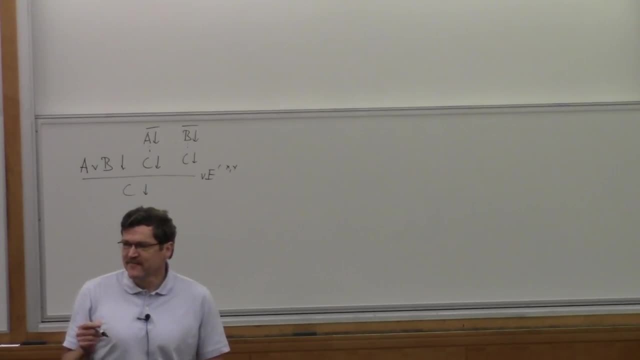 Okay, So I worked on it for a few minutes. and, yeah, you worked on it. What was your answer? Okay, So do you want to tell me what you thought about? Yes, because these are all down, or everything has to be on the left, right, so that's okay. 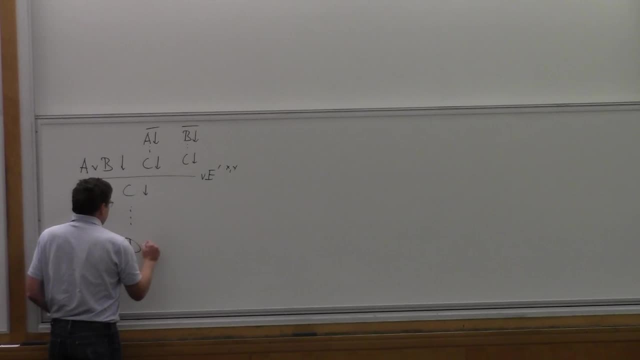 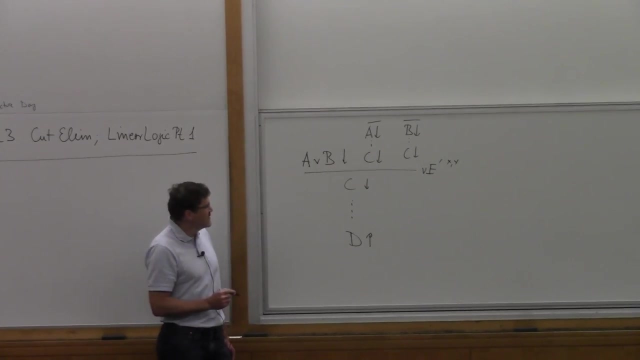 But this happens in the context of a bigger proof, right Where you're trying to do this right. So that's where the D comes in. okay, So then, Okay. So then now, what do we conclude from there? Okay, Okay. 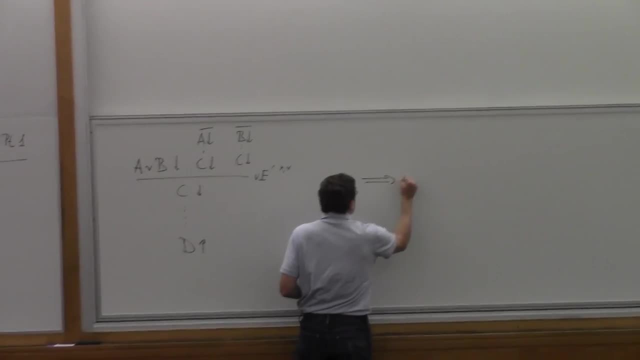 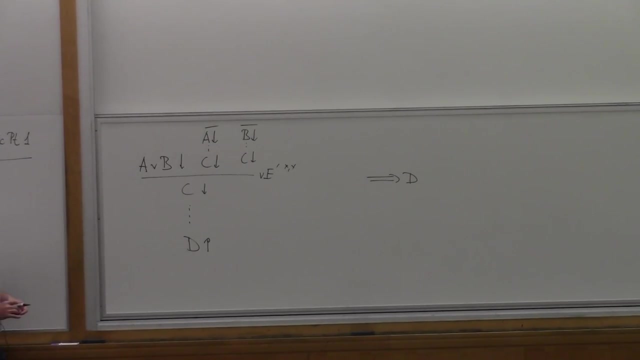 So we, we should have a sequence, Something that's略 Okay. So we, we should have a sequence, Something that's略 somehow, where we have d on the right-hand side, right, And now it starts to break down right. 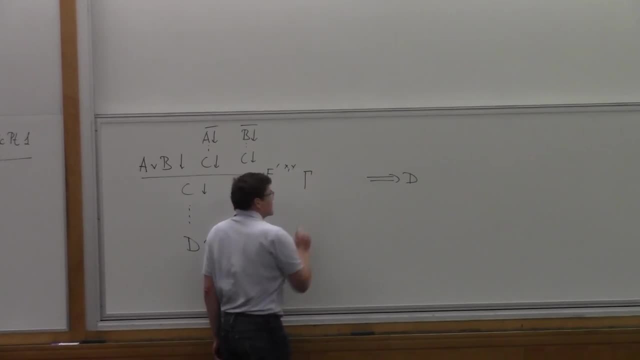 OK, well, we always have a gamma. OK, So far, hardly any controversy can erupt. OK, Now we're supposed to be able to use a or b, So that should be over here, right, OK, so we don't really when we start. 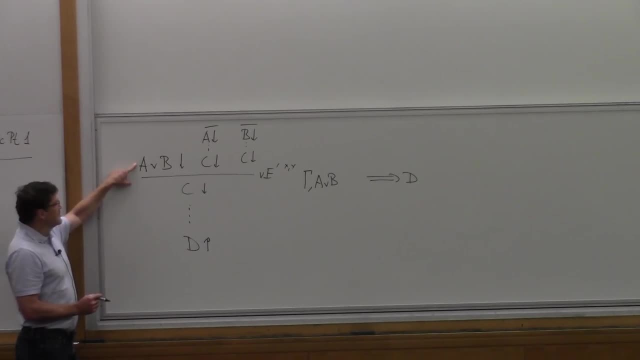 we shouldn't have anything else, should we? We should just have a or b, because we want to apply elimination to that right. OK, so, all right. so then, what can we say about here? OK, well, we still have a or b, right. 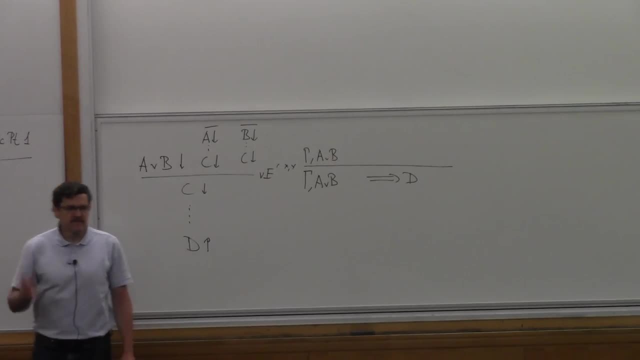 That's our principle: Once we have something, we'll always have it for the rest of the proof. So that's another question. There's two branches, so we should probably have two premises, all right, In both branches. OK, so now it becomes really tricky, right? 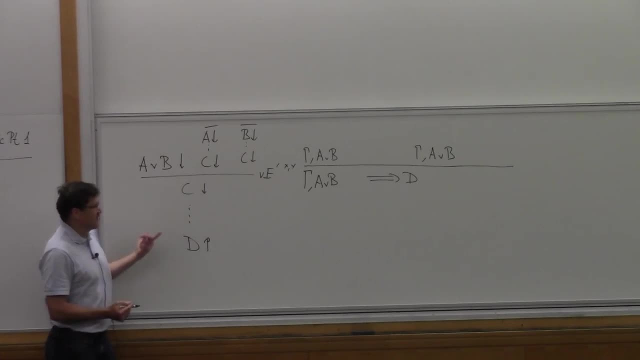 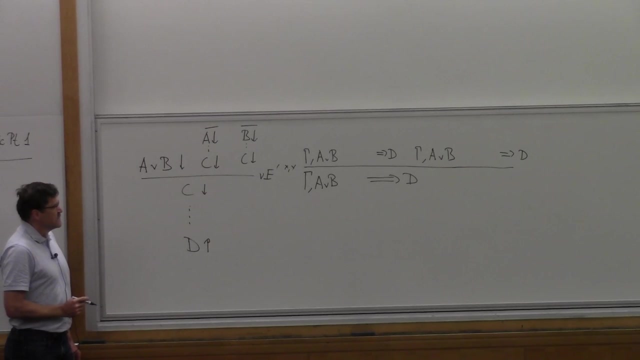 I want to say: we're still trying to prove d because c is on the left-hand side, So somehow we should still try to be proving d, OK, so at this point I got stuck because, well, maybe in this branch we should have a right. 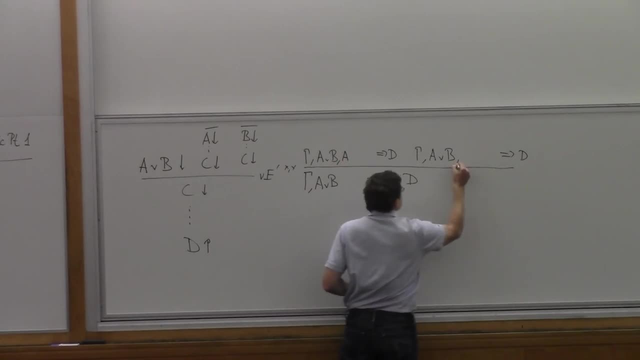 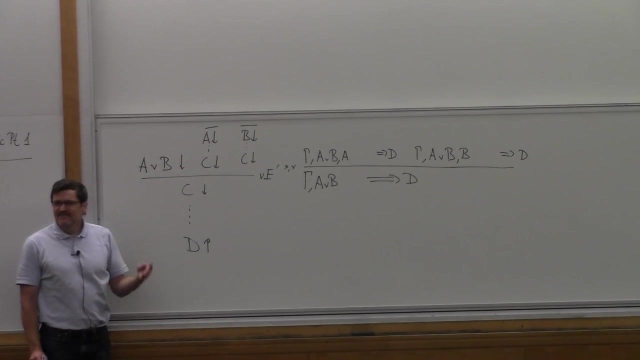 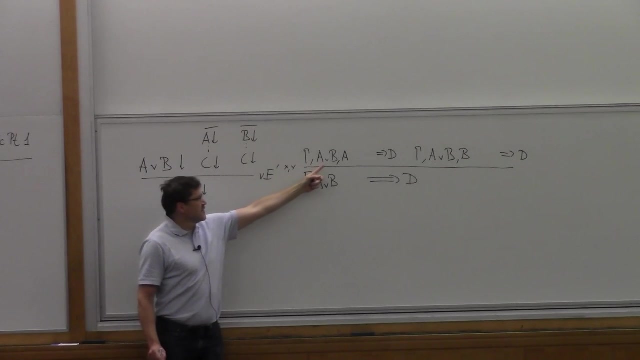 So we should have a as an assumption And here we should have b as an assumption. But how do you represent the fact that from these assumptions we can deduce c as a conclusion? Because the only thing we're allowed to write on the left-hand side is things that we know. 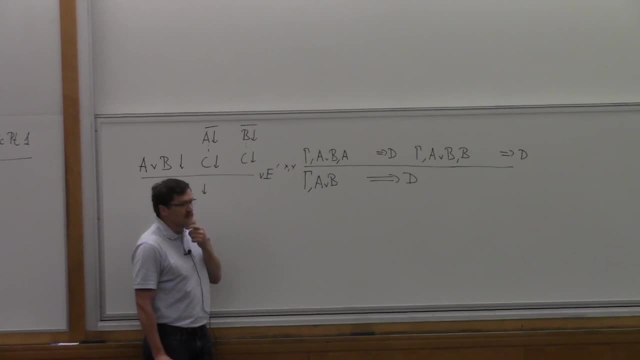 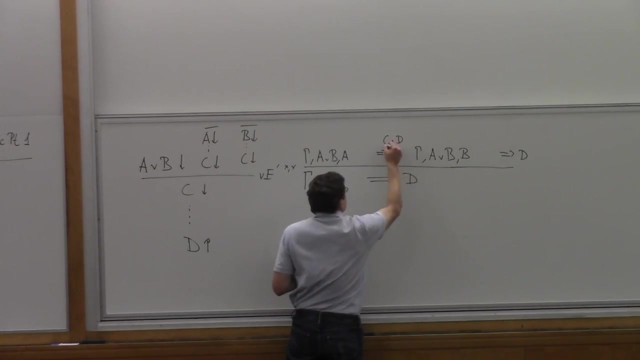 We could write c and d here, But that would mean it would be an up arrow right Constructing a verification of it because it's on the right. OK, so that doesn't work. Not c: OK, Maybe if we're a classical, and also then it's not really. 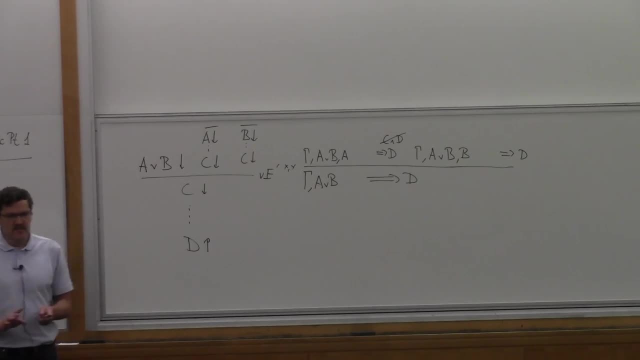 clear what we mean by on the right and the left. So maybe there's an out there. I don't see it, So I came to the conclusion at this point: OK, there is no sequent calculus rule that expresses that. OK. 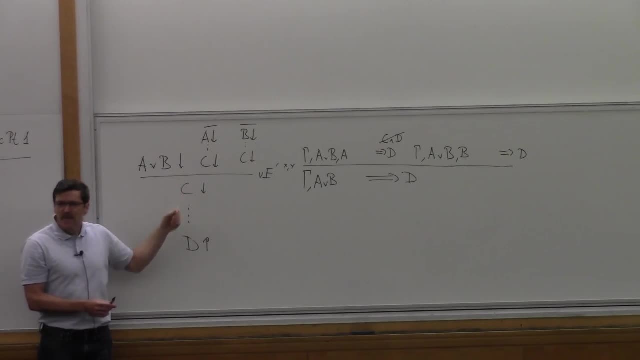 And so that means that this rule is a bad rule, right? Because for all the other rules we have a perfect correspondence. They have a certain shape and form. There's a logic to it, right, That you only work with introductions from below. 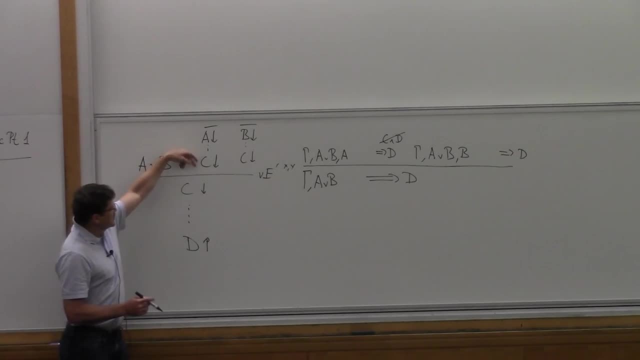 eliminations from above. OK, And whenever you have a problem, you have a proof that you're trying to construct. you're almost trying to construct a verification at the bottom, rather than that something can be used. So we would need to generalize our sequent calculus. 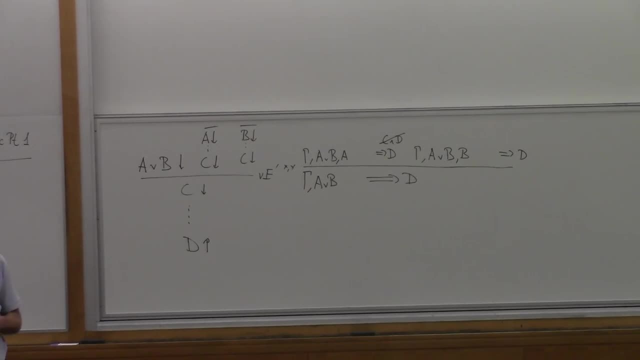 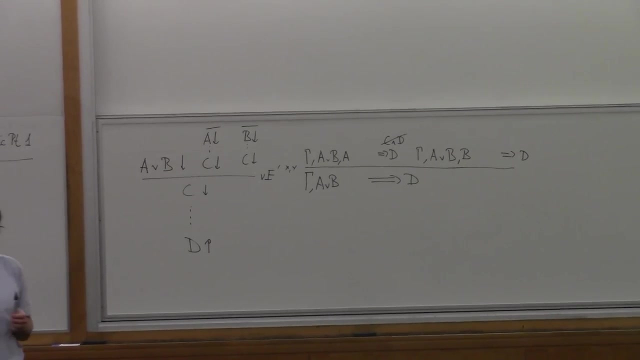 to something different in order to be able to capture the contents of this rule on the left. OK, So is that the conclusion you came to? Yeah, I kept thinking it doesn't make sense to be able to. Yeah, I hope there was a different answer. 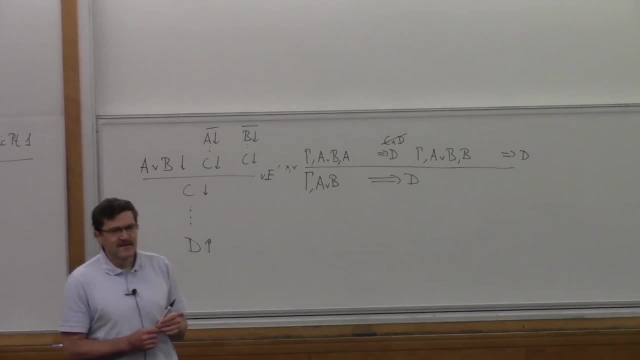 No, no, You got the right answer right. There is no rule in the sequent calculus, so we'd have to generalize the sequent calculus to figure out how to do it right. So, OK, Good, So you know. I'm collecting reasons why this rule is bad, right. 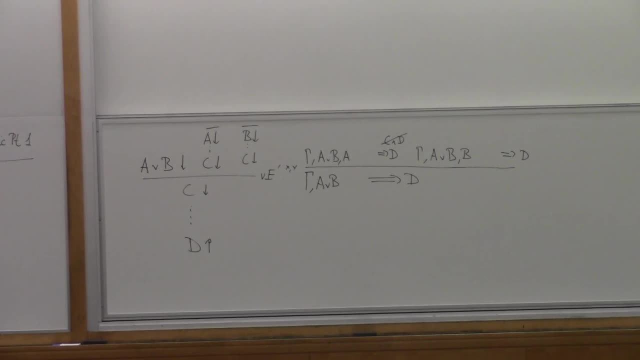 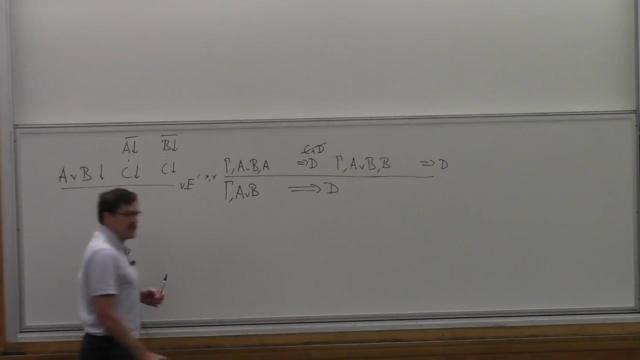 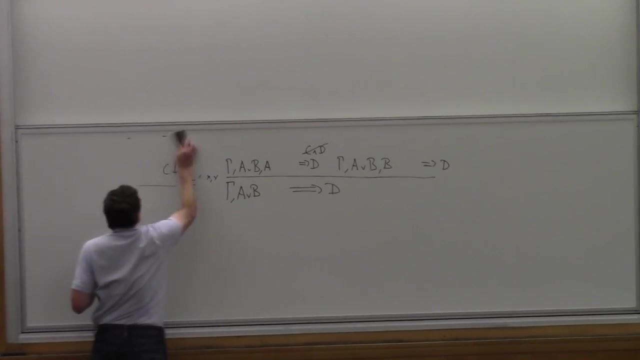 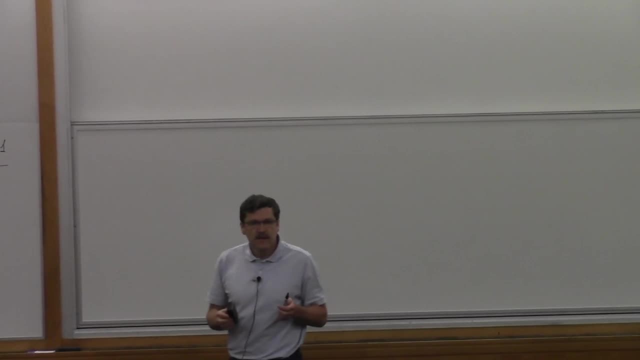 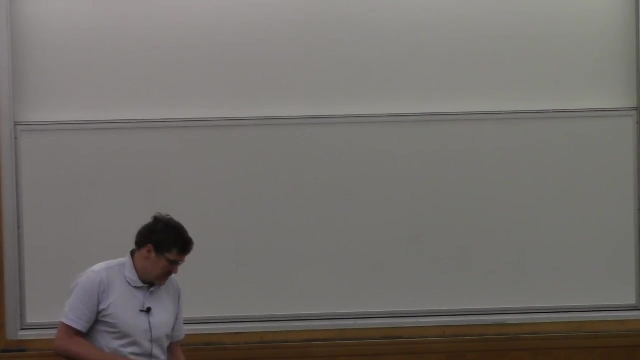 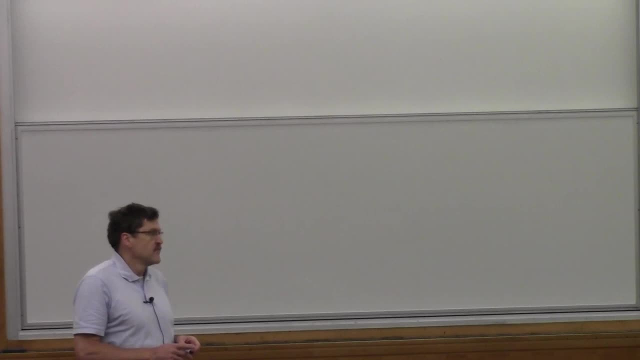 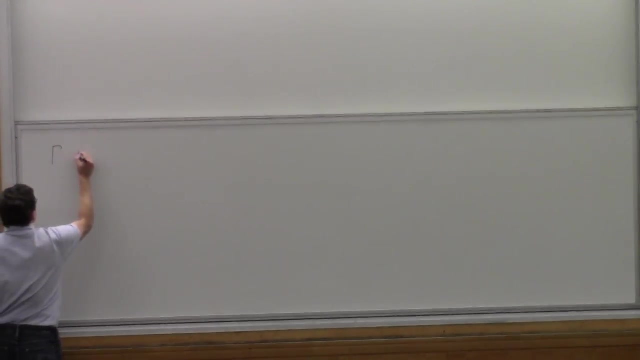 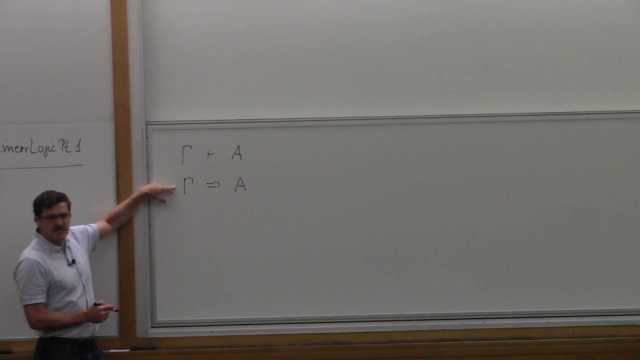 OK, OK, OK. so what shorthand I mean? so the reason: OK, so so in these lectures, and also in Bob's lectures, you use this notation for natural deduction, and so I felt compelled to make a different notation so that these things are distinguished. 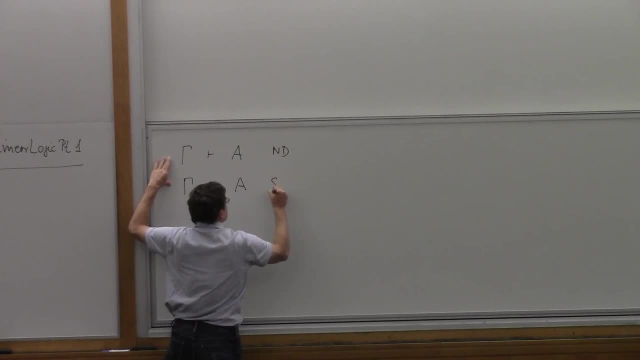 So this is natural deduction and this is sequent calculus. And I could equally write royal turnstile here, OK, but then I would need to distinguish some other way. then I would write above the turnstile. OK, this is natural deduction. 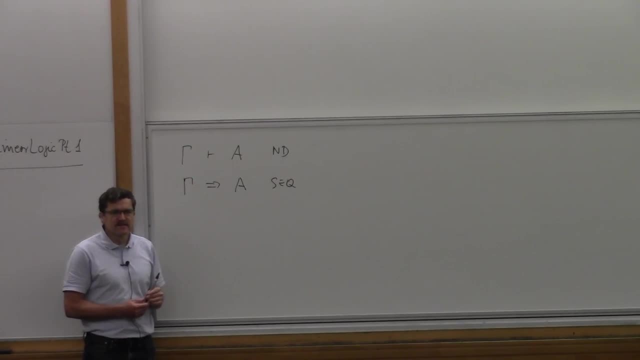 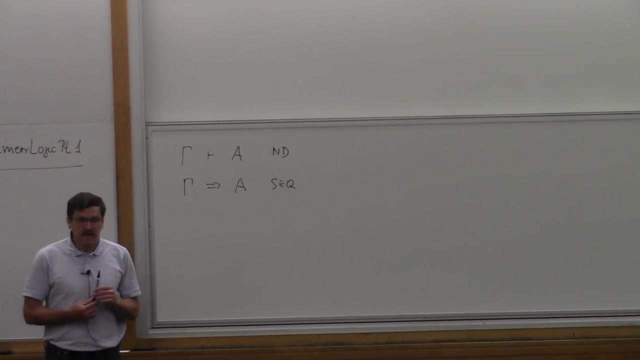 this is sequent calculus and that gets tedious. OK, so there's no deeper meaning to it than that. OK, Yeah, Yeah. What was the source of the rule that you used in that game and you found it could not be? 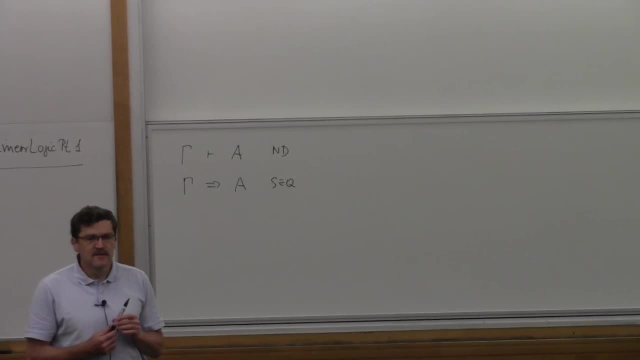 a student. but it was a student. A student, No, No, I mean, you think about the rules you try to figure out and then you know, the question always comes up: well, why, what about that rule? OK, could we have that right? 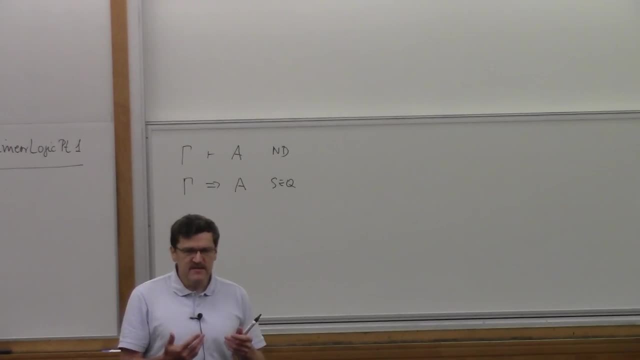 And it doesn't seem to fit. In some ways it fits because it's still satisfied the subformula properties, but in other ways it doesn't fit. And one way to see that it doesn't fit is that it doesn't have a corresponding sequent. 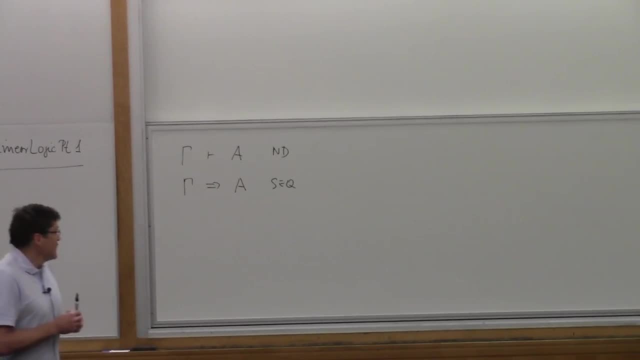 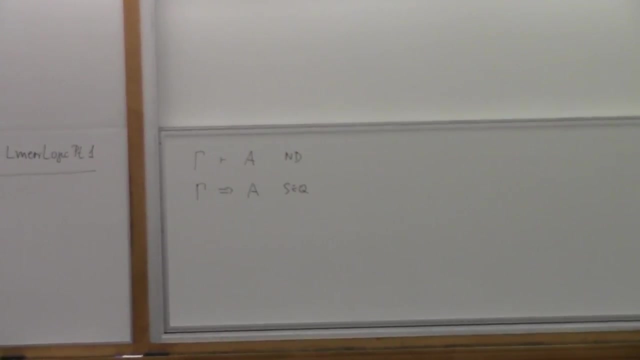 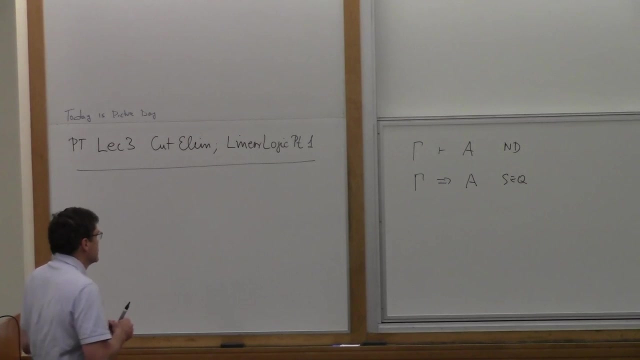 calculus rule. yeah, All right. yeah, For the temporal logic sequent calculus. it seemed like there were some. are there any arbitrary choices? in which ones were down arrows and which ones were out errors? OK, are there arbitrary choices? OK, so let's think about that. 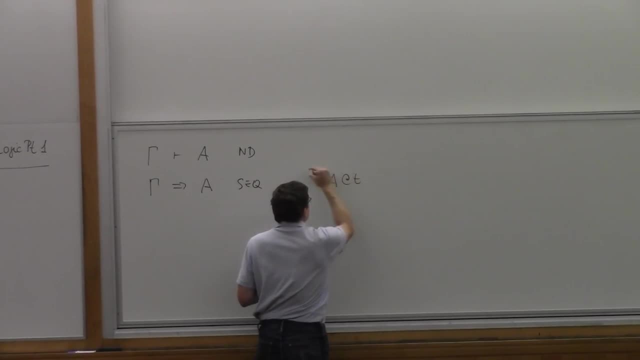 So to prove circle A at type T, you have to prove circle A at time T plus 1.. OK. so question is: should the OK this be up arrow or down arrow? It should be an up arrow. Why should it be an up arrow? 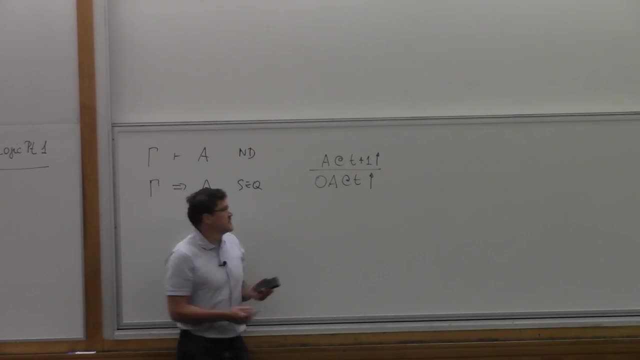 Yeah, that's kind of a second order reason, but there's a very simple reason. This is an introduction rule, and the introduction rule constructs verifications, and constructing a verification means that you have to go from up to up. And what's the elimination rule? Well, 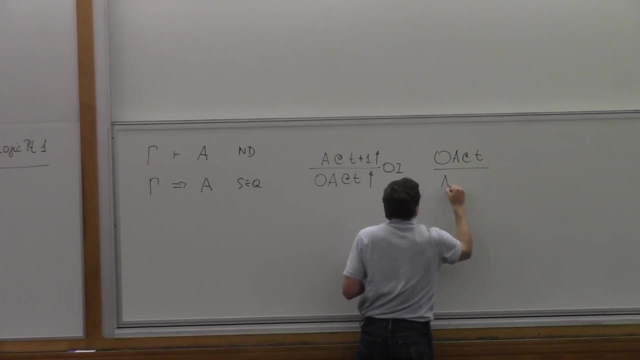 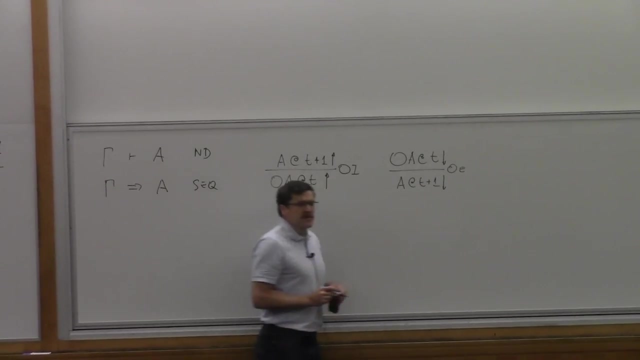 if you know a at time t, then you're allowed to circle a at time t, a at time t plus one. This is the elimination rule. So what should the arrows be Down? because this is how we use the knowledge of circle a, and so elimination rules are the. 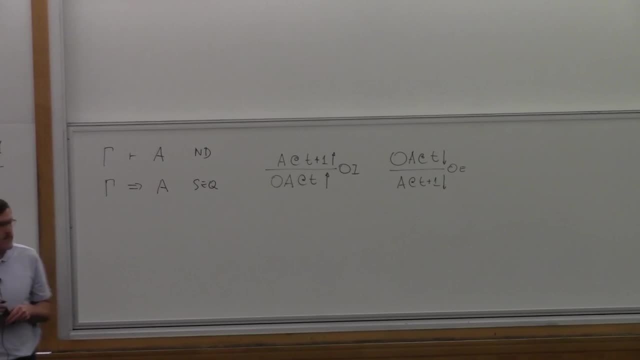 down arrow. So I don't think there's a down arrow. So I don't think there's a down arrow, So I don't think there's any ambiguity. Okay, so if it's an up, that would be wrong, because to prove a you would have to invent a bigger. 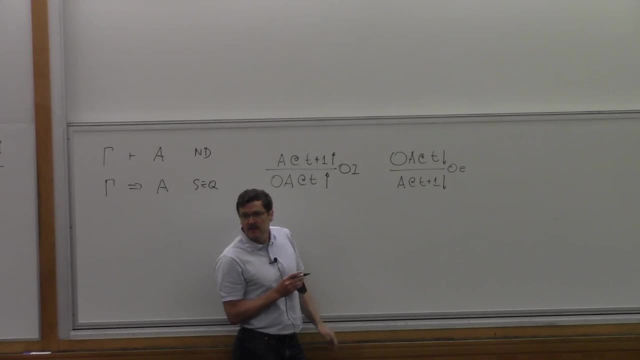 proposition, So the premise would not be a subformula. Yeah, so the propositions here is this and this. So you couldn't use this as a verification rule, because you'd have to. you know, the meaning of a would depend on the meaning of a larger formula. 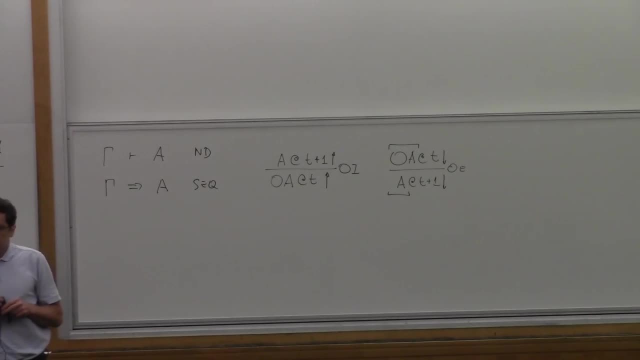 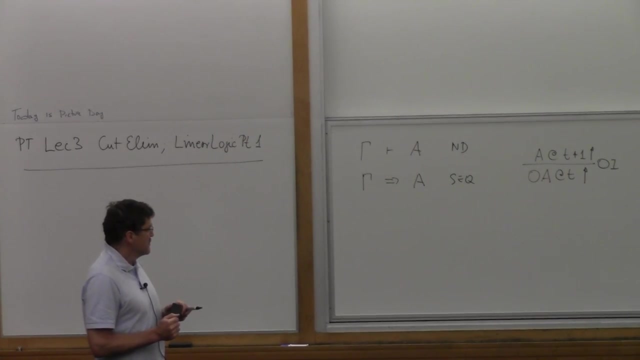 So you can't do that. So you can't do that, So you can't use the up arrow there. Okay, All right, So okay. so I want to do two things today. First, yeah, Well, what if you made it the other way around and then you knew that t was going down? 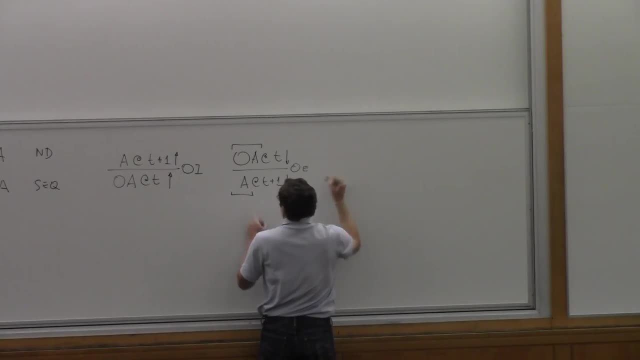 The one on the right would be up there and the one on the left would be down there. I mean, these ones would be down arrows. Yeah, Okay again, if a down arrow, you need to assume you know that, and then this has to be a subformula. 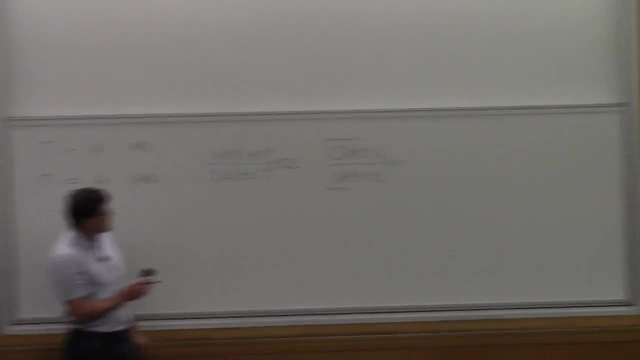 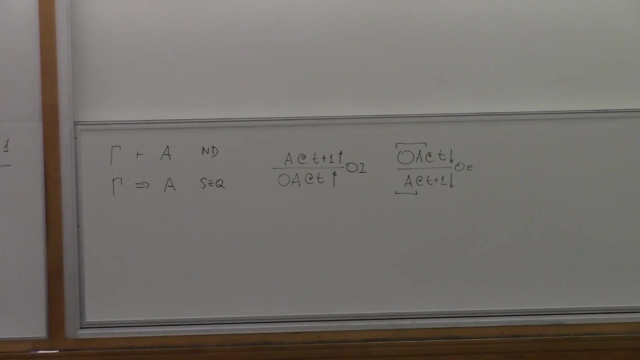 that it would not be the case. But, yes, the number gets smaller. Oh, the number gets smaller. Well, the judgments: when we consider these directions, we don't consider the judgments. We consider whether we break down the propositions because we want to use the rules to explain. 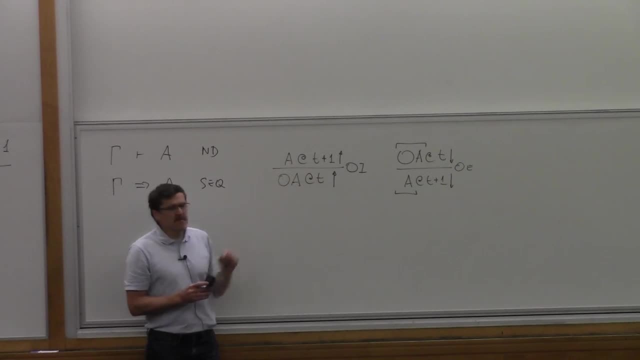 the meaning of propositions. Okay, so the fact that time gets smaller, that might be something that we don't know. It might be something different. I haven't thought about how that might fit. It's interesting, There might be something to be said, but I haven't thought about it at all. 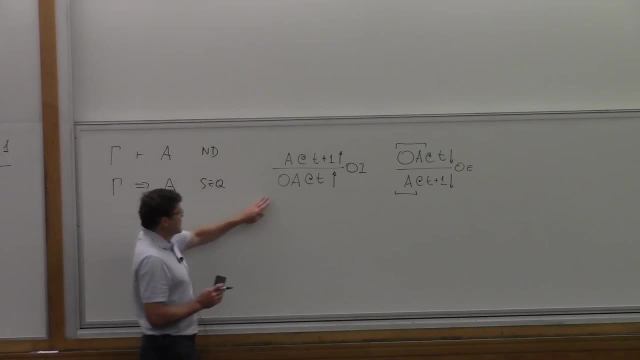 So we're just thinking about when we have these rules there- introduction, elimination, those four propositions- and we focus on this part. okay, All right. so what I want to do today is: first, I want to actually talk to you about 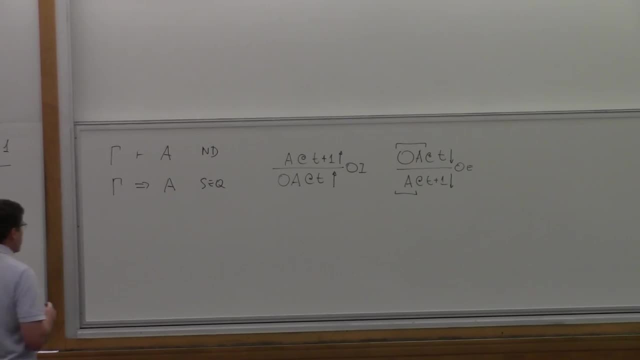 how to prove properties about systems and complete this kind of a picture that I started to paint about how sequence calculators work. You can see that these two propositions, which were in the very beginning, we already are in the very beginning on this part, right. 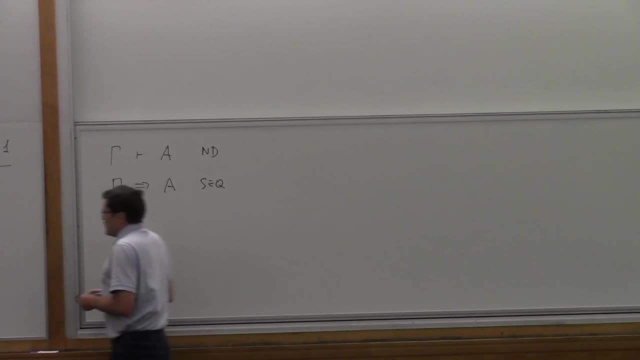 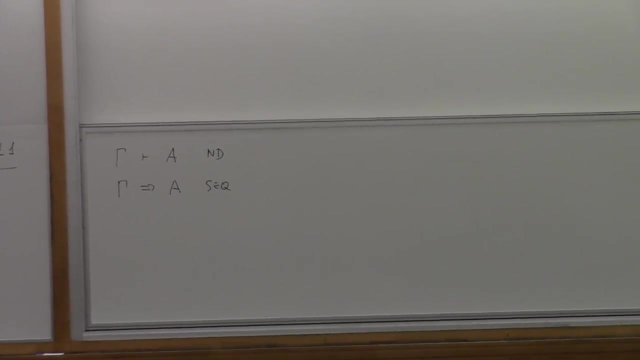 So we have written them into owes methods so we can see which ones are Gaussian right now and which ones are maybe two hundred twenty dimeth. Now let's see how we can get the total vector for which we think we've made Jack Holmes equations. 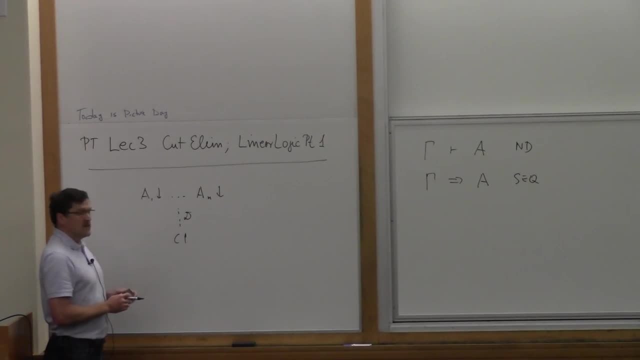 So let's say, say that the sum of: if I don't tune this out, then there are just what I should be doing right here. Okay, which I'm going to write like this for these verifications. So I'm going to have a up here. 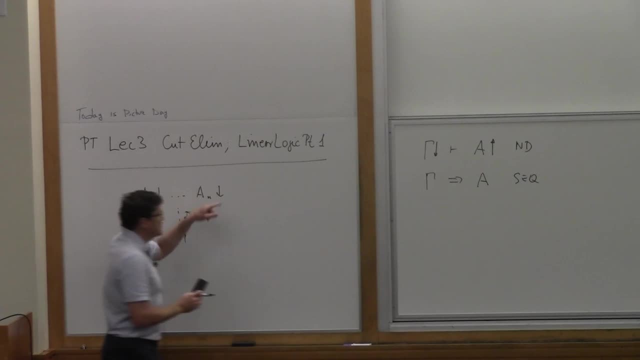 And this is gamma, And every formula there is annotated with one of these down arrows because we're looking at verifications. So, because this is a hypothetical judgment and this is our notation for hypothetical judgments, it's completely consistent. It's just a one-dimensional way of writing things. 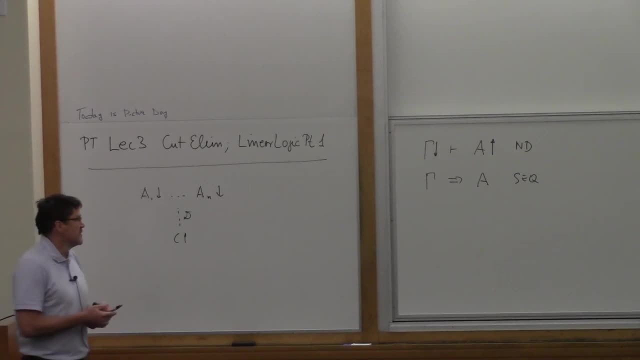 which are two-dimensional over here, So it just makes it easier for me to write, But it's exactly the same as this, So there's no semantic difference between: And sequent calculus are still right like that. So now what I'd like to prove is that verification. 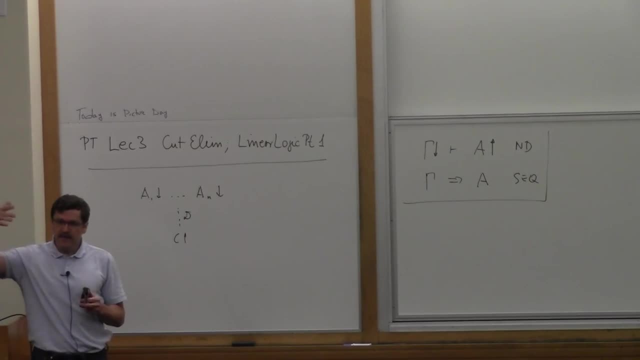 and sequent calculus are actually the same. So this intuition that I had when I constructed the sequent rules, I want to express this as a theorem and verify that it's really true. I didn't make any mistakes. So there's two directions. 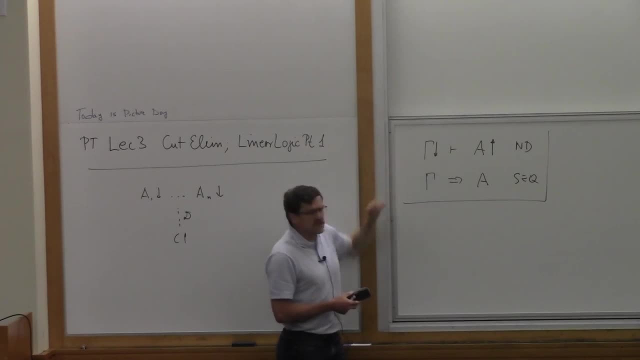 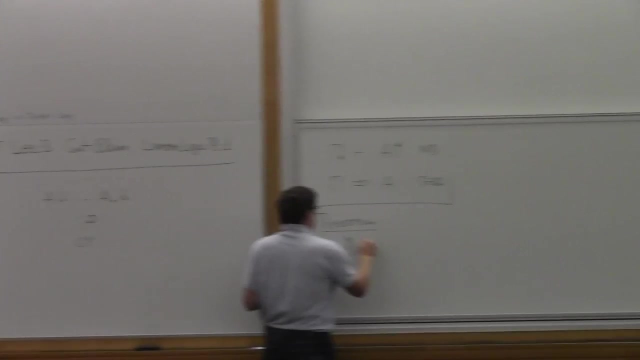 One direction. if this holds, then this And the other direction. from here you can go back to here. So I'm going to just do one direction And what I want to prove is the theorem. So if gamma down proves A up in natural deduction, 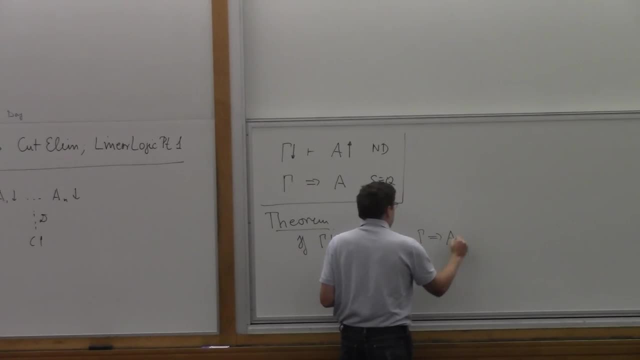 then in the sequent calculus we can prove A. So now, how do you prove theorems? for complete theorem It's only بال, And we do that by considering all the possible cases, the way the proof could be constructed. We have to make sure that we know. 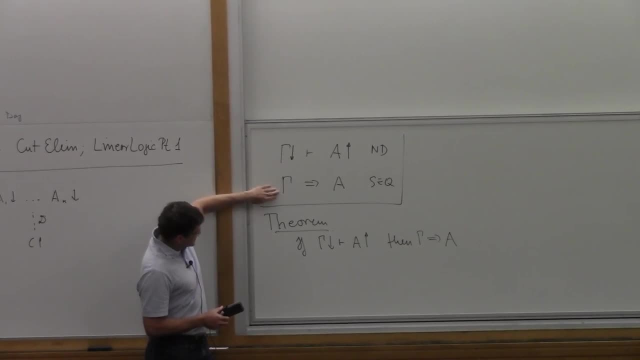 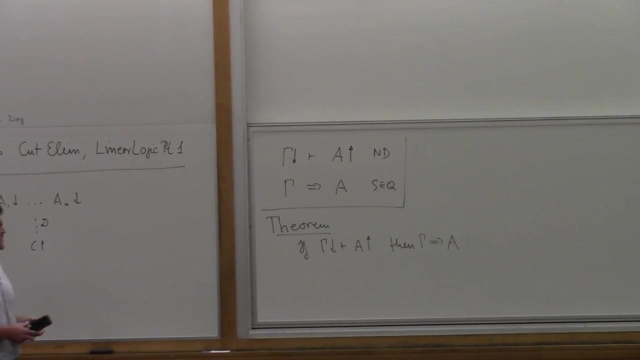 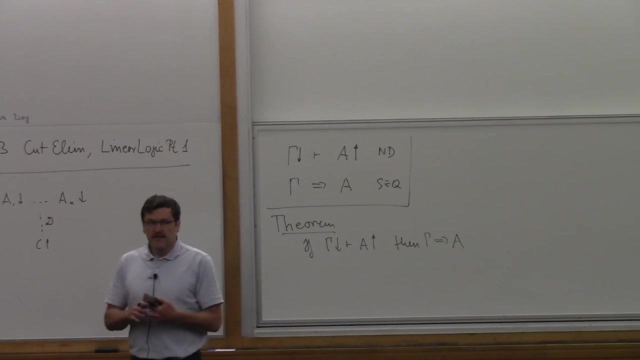 how to construct this proof from the parts that we have here. So I'll walk you through a couple of cases and then we'll see how to actually go about how this kind of thing works, just so you see how to reason about the system globally, right. 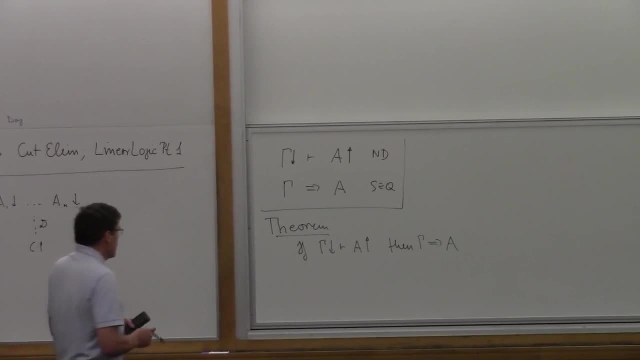 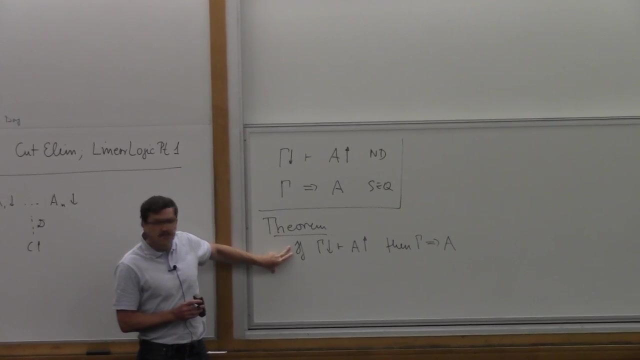 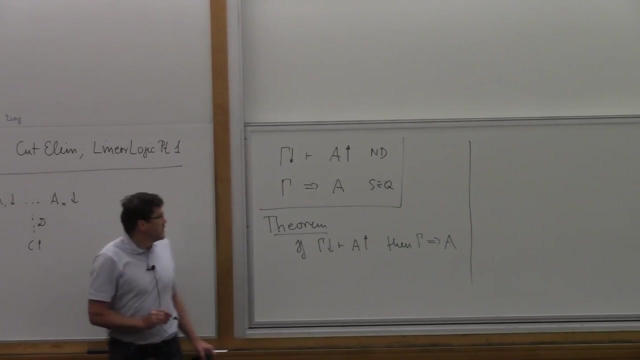 We have done these local tests so far, but now we're actually doing something global, because we're fixing now our system here entirely with all the connectives, and then we're trying to prove that. okay, All right, so Okay. so there's a second theorem. 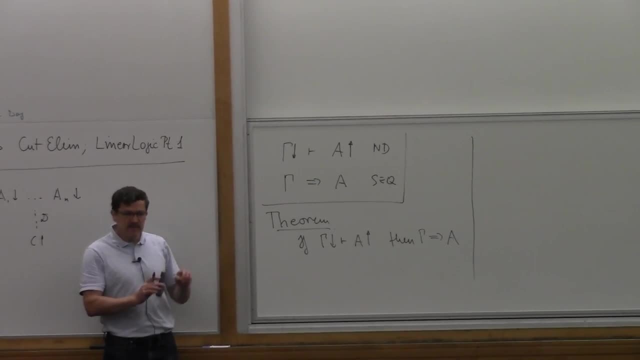 which goes back from here to here. but I don't want to prove that. I want to, you know. Otherwise, I could spend, of course, a whole lecture just showing you how to prove these things, but I just want to focus on one. 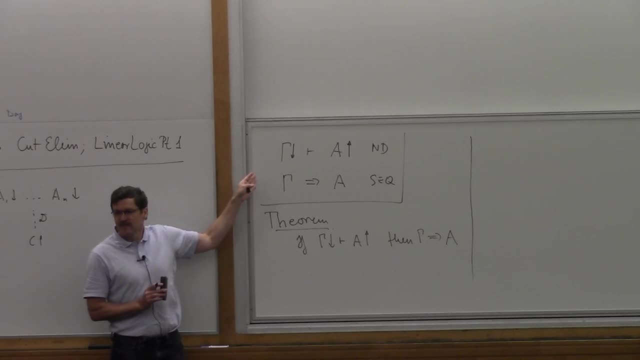 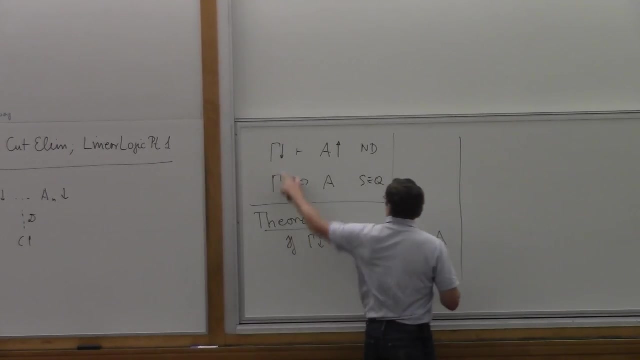 This from here to here is the easier direction, so I'm going to the more difficult one, okay, All right, So now we're looking at the possible cases for this. Okay, so let's give this thing a name. Let's say: this derivation is: 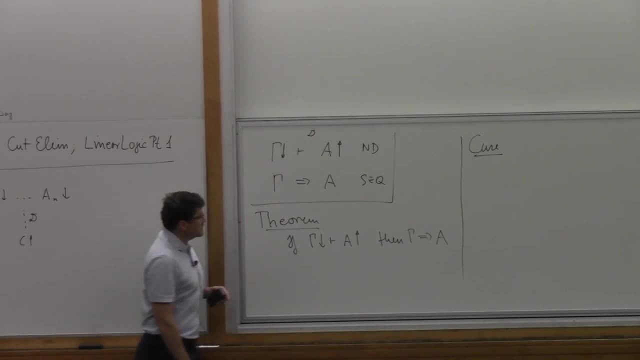 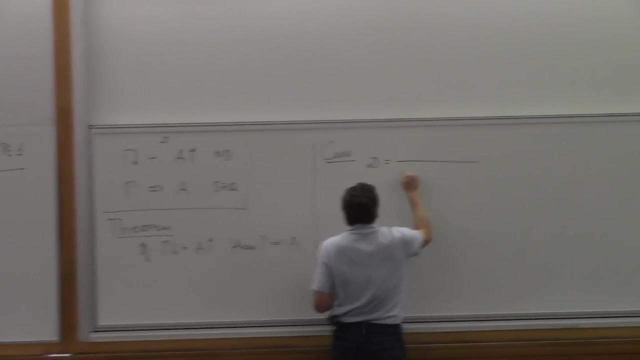 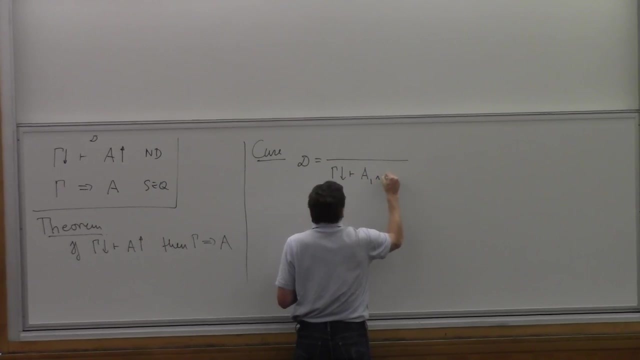 Well, okay, let's say it's d, Okay, Okay. So one possibility for d is that it looks like this: We have gamma down proves a1 and a2, and we have a verification of that, because in gamma down we have a verification of a1,. 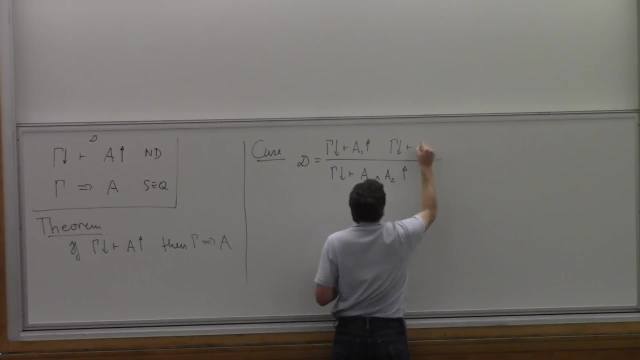 and in gamma down we have a verification of a2, and let's call this derivation here d1 and this derivation d2, and this was done by end-introduction. Okay, So when we're doing induction over the structure of a derivation, 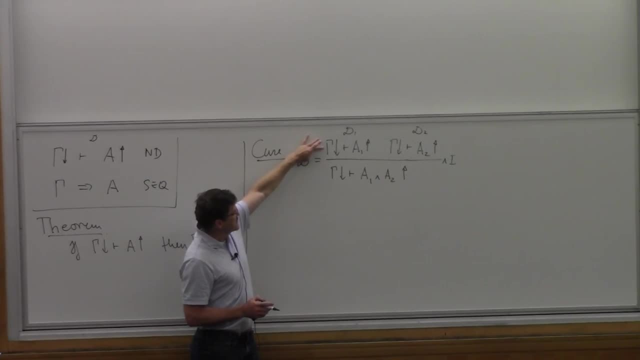 okay, we can apply the induction hypothesis to the sub-derivation. so we can apply the induction hypothesis here and the induction hypothesis here. right, because we're considering, you know, the structure of the proof, structure of this derivation here. 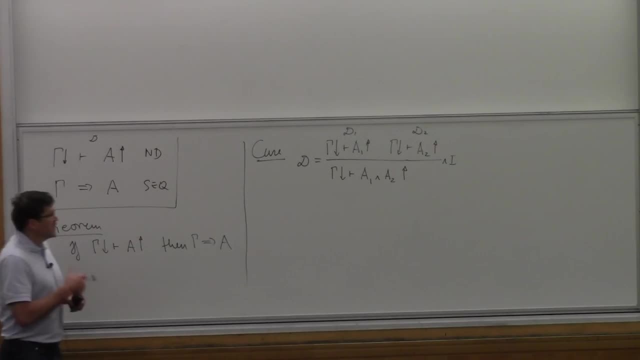 as something that we do induction over. Okay, So if we apply the induction hypothesis to d1, what do we obtain? Yeah, So what we get is from gamma we can prove a1, and this is by induction hypothesis on d1.. 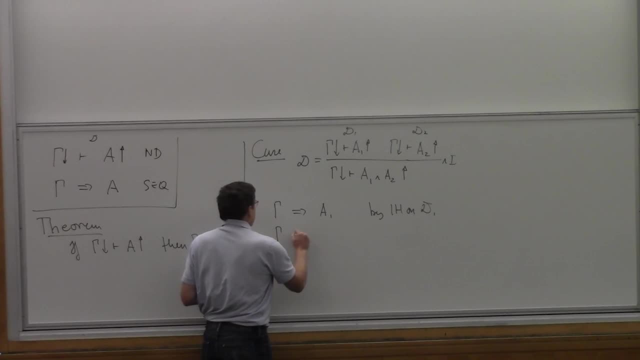 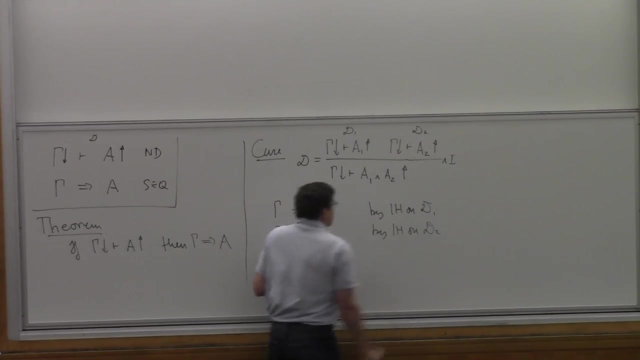 Okay, We can apply the induction hypothesis to d2, so we get gamma proves a2, and we get this by induction hypothesis on b2.. Now, what do we have to show in this case? We have to show that gamma proves a1 and a2. 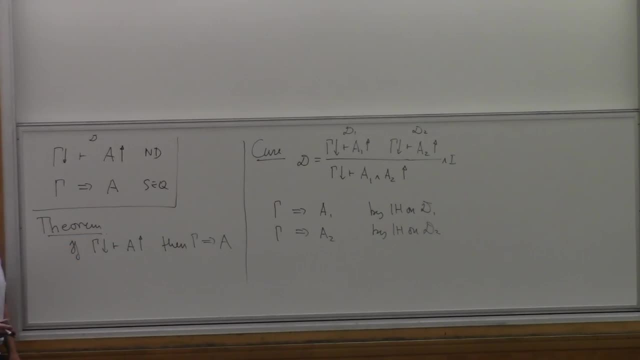 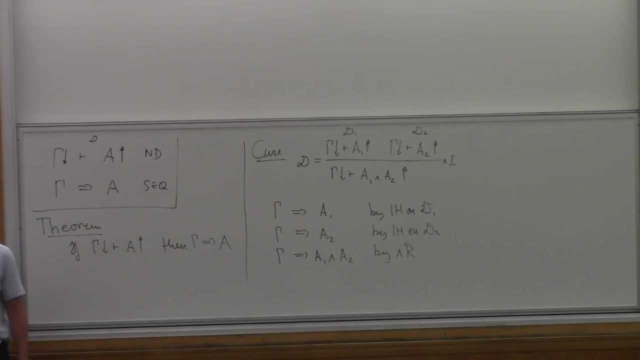 in the sequent calculus. Okay, how do we get that? Yeah, So then gamma proves a1 and a2 by the right rule for and in the sequent calculus. Okay, And all the right rules follow the same pattern, all the introduction rules, I should say. 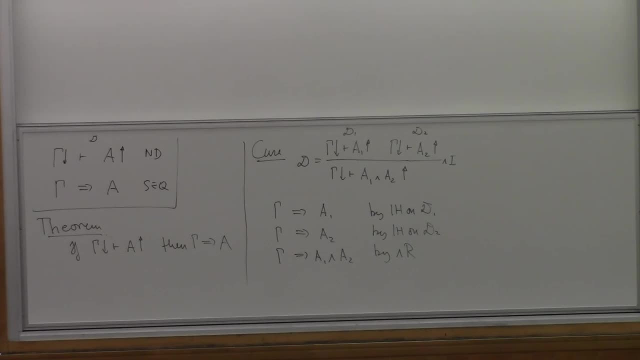 follow the same patterns because if you remember globally what you did is introduction will correspond to right rules and elimination rules correspond to left rules turned upside down. So the cases when, the cases in this proof, where we use introductions, they're going to be fairly easy. 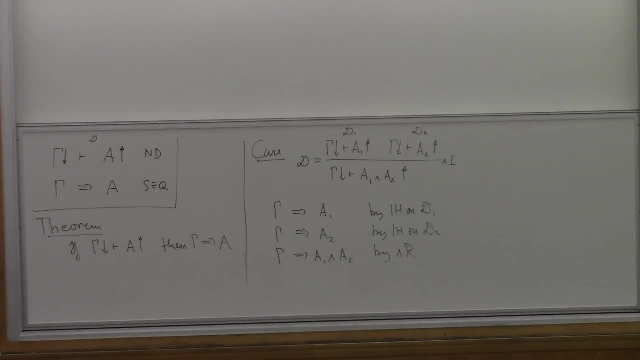 because they all follow in the standard way, because the rules are mirrored exactly. Okay, Everybody on board with that part of the proof? Okay, Okay. So where do things become with elimination rules? obviously, And in fact, our theorem doesn't say anything. 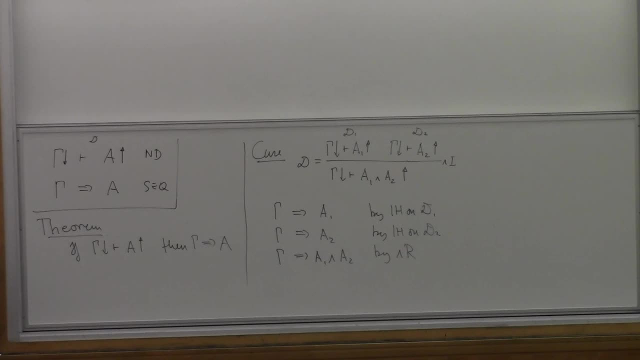 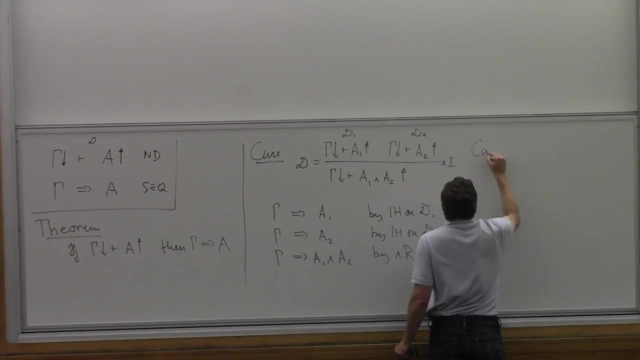 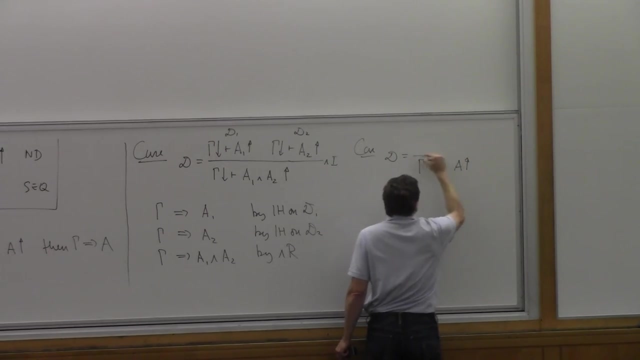 about elimination rules, right. So at this point we realize our induction hypothesis is not going to be strong enough because, when we come to this case, d is gamma down proves a up. because d is gamma down proves a up. because gamma down proves a down. 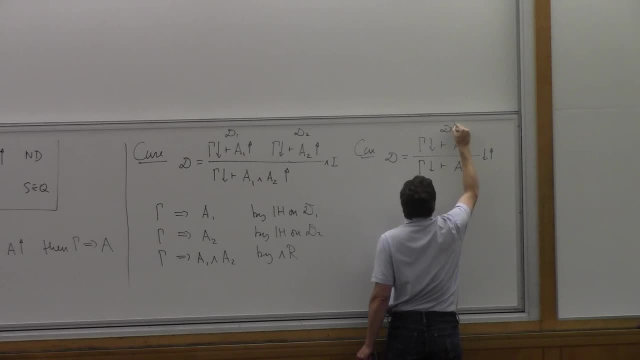 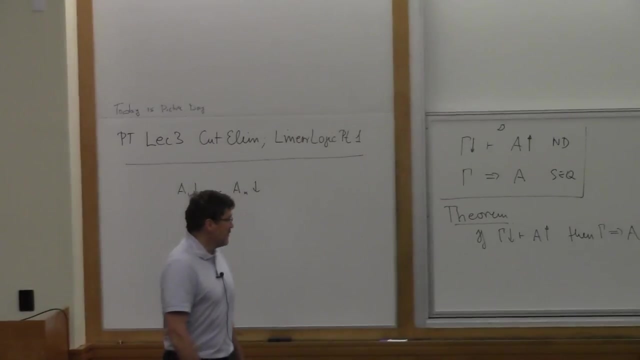 and this is some other derivation d prime. Okay, We can't apply our induction hypothesis to the sub-derivation because it's a proof of a down and all we know here, all we have stated so far, how to handle a up. 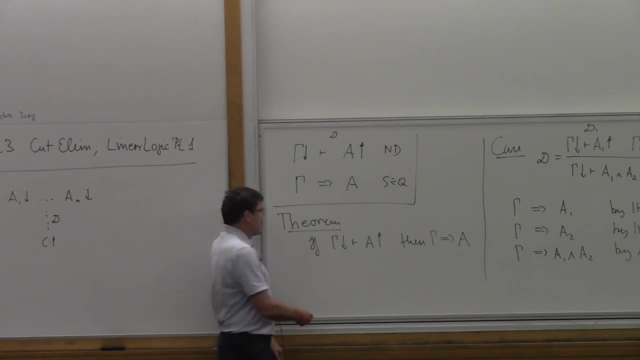 Okay, Clear, Okay, so we're stuck. Okay. so then what we do is: Okay, that's the first part. We need to generalize our induction hypothesis. We need to say something about what happens with a down. okay, 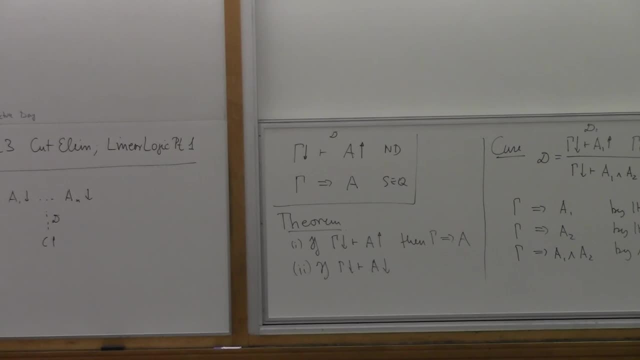 All right, and now comes the really creative part in this kind of proof. okay, What is the right part of the induction hypothesis when a down holds? okay, Now, the very first time I did this kind of a proof some years ago. 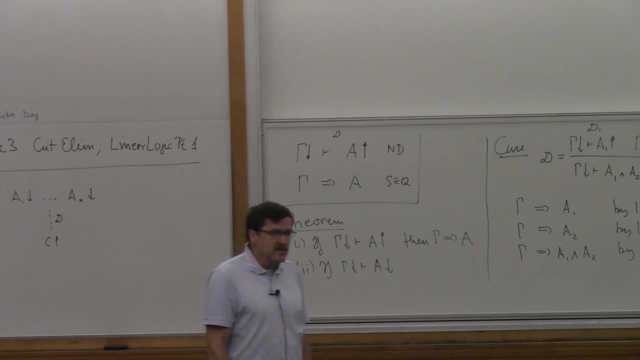 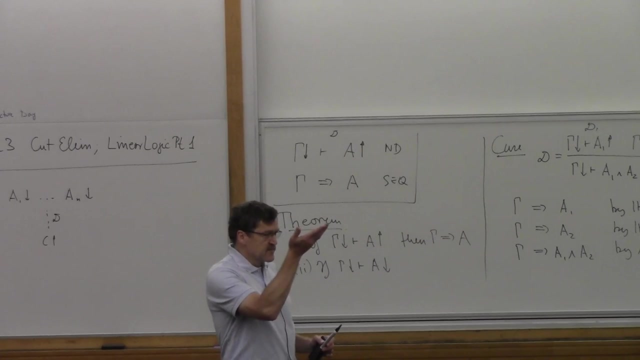 it took me many hours to figure out how to do this. It seems completely obvious. right, Because we translate the right rules to right rules and the elimination rules to left will turn upside down. right, And we were very careful to do it the right way. 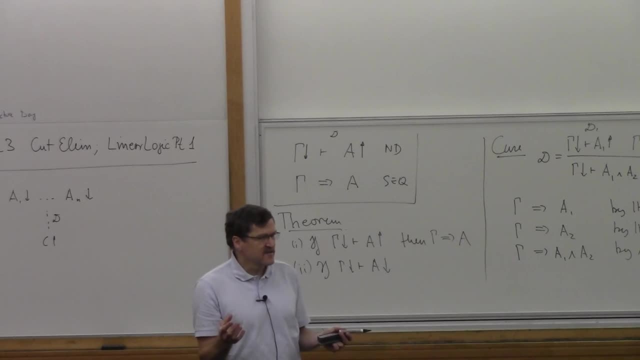 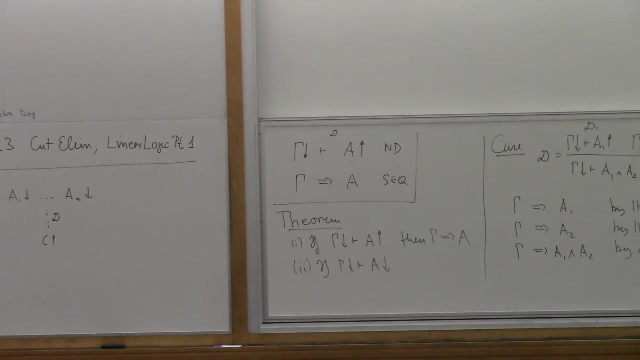 So it should be very, very simple, right, But how do you prove it? by induction, Okay. does anybody have any thoughts about how to do that? Yeah, Yeah, Gamma comma a- proofs top. Okay, so the gamma comma a, I agree with. 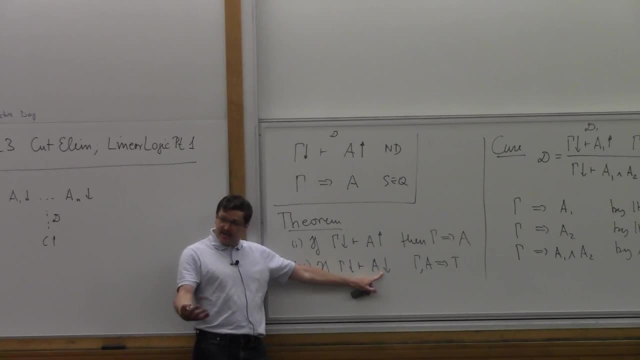 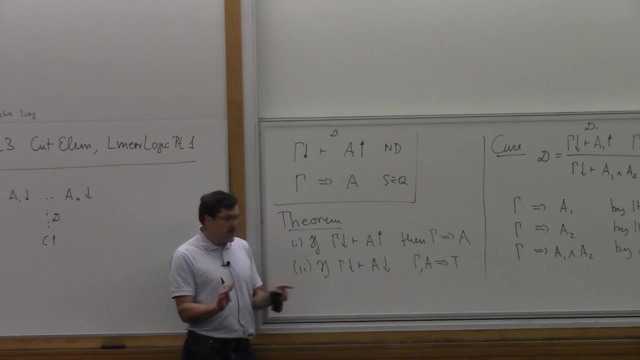 And the reason it has gamma comma a: because a is down. in our translation, something with down ends up on the left-hand side, So we already know that much. right, We have to talk about a on the antecedent of the sequent, okay. 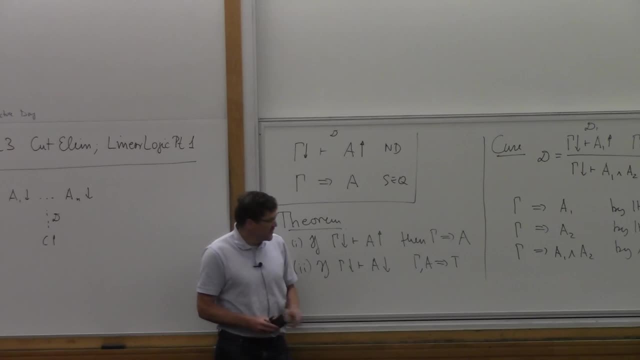 Now the gamma top. okay, I don't believe that, because you can. You can always prove top, no matter what. your assumption is Okay, so that's Okay. so we know the gamma a, But what do we prove on the right-hand side? 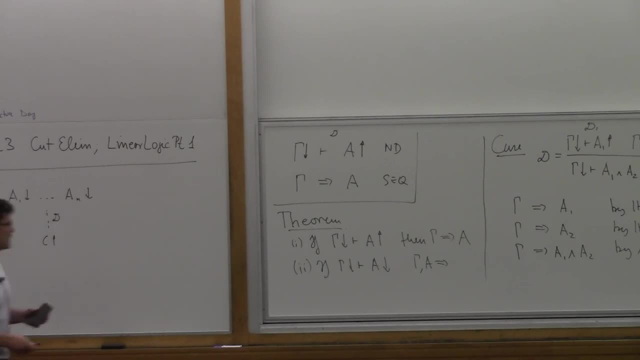 Yeah, Okay, So unless you have seen the proof? okay, you just shortened my five hours trying to figure this out into ten seconds. okay, Because this is indeed Yvette and this, Then gamma, proof C: Okay, so what we're saying here is that. 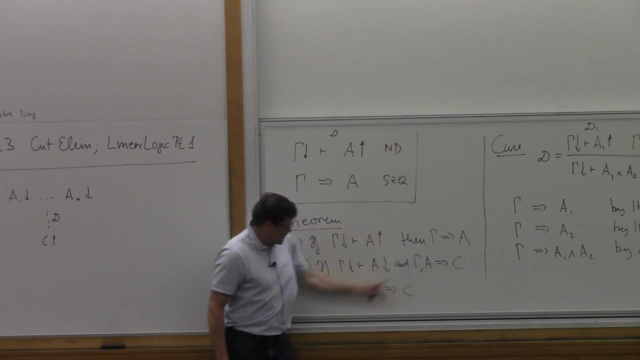 if this gamma justify the use of a, then this proof of C doesn't need to depend on a, because gamma justifies it. Okay, All right, so let's try to do See if that works. Okay, let's see if it works here. 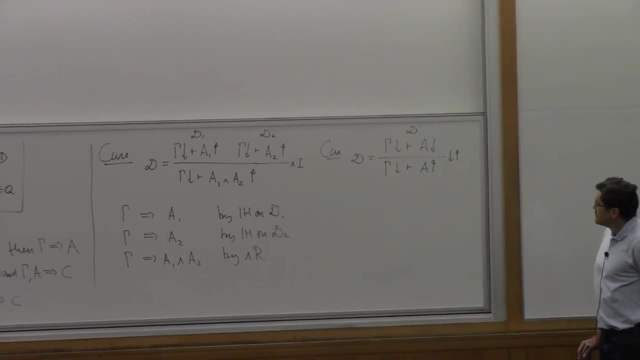 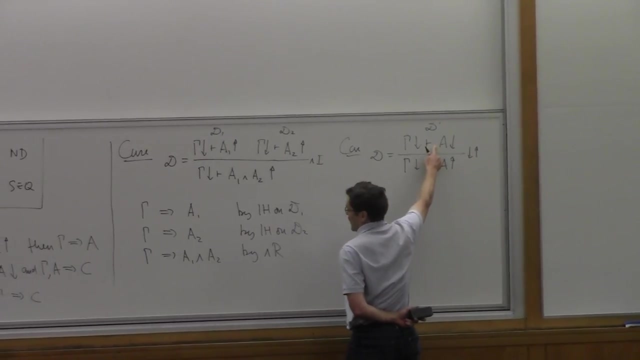 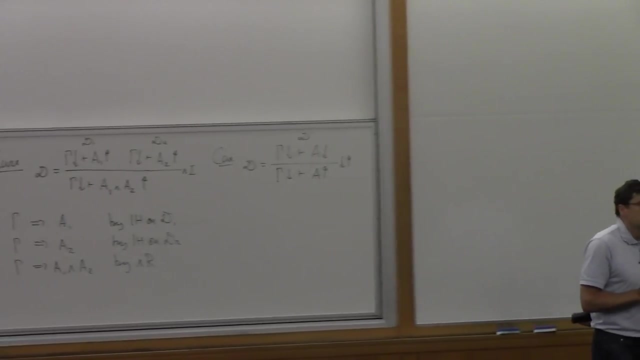 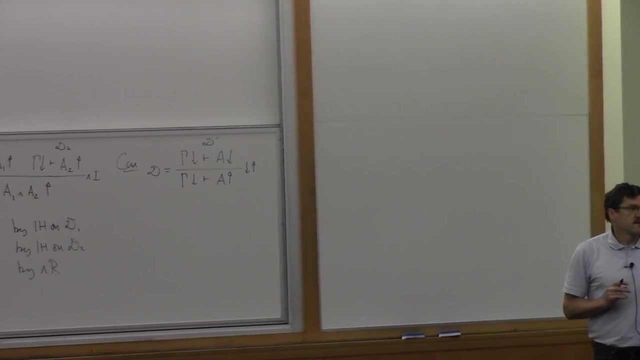 Okay, so first. So to apply the induction hypothesis, we should have some proof of gamma, together with a proof something. So what would that be Actually, before we go there? in our translation, what did the down-up rule translate into? 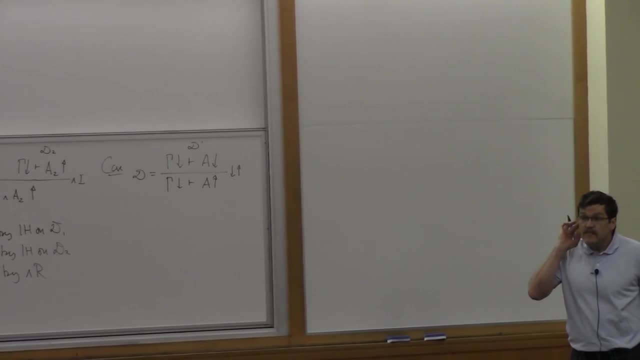 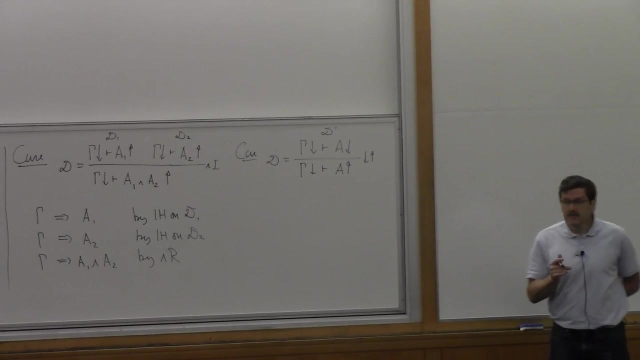 Anybody remember this? The what, Yeah, the variable, which we actually call the identity rule. So remember this. The picture was this. It doesn't hurt writing this down: We have eliminations here, introductions here, and they meet at the down-up rule. 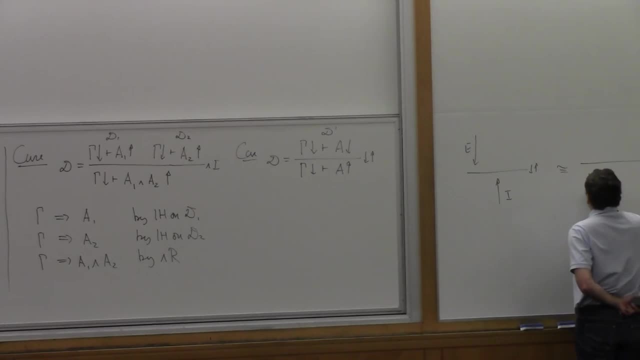 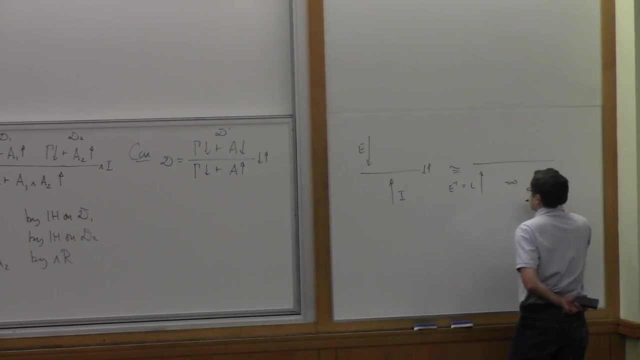 And this corresponded somehow to like this, and we had the left rule, which were the inverse of the eliminations, And then the secret arrow in here had the right rules, which were equal to the introductions, And this was the identity rule at the top. 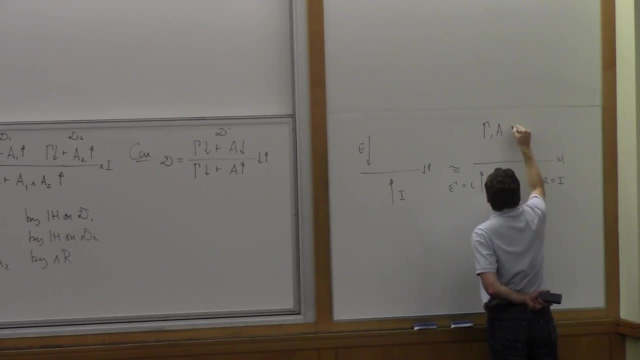 And the identity rule said: if you have one assumption A, we can conclude A right. Okay, which is called the variable rule. in natural deduction We call it the identity in the sequence calculus. Okay, so we should use the identity rule here.